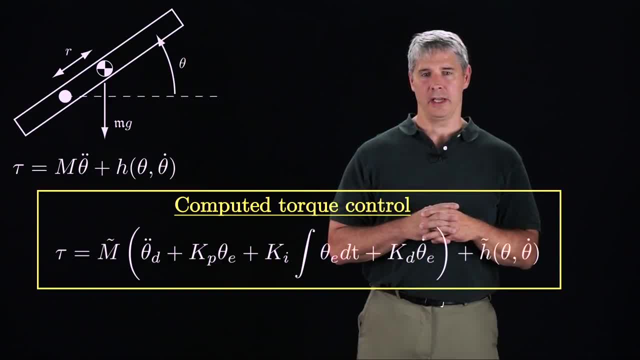 Because of this possibility of instability raised by integral control, integral term can be eliminated. 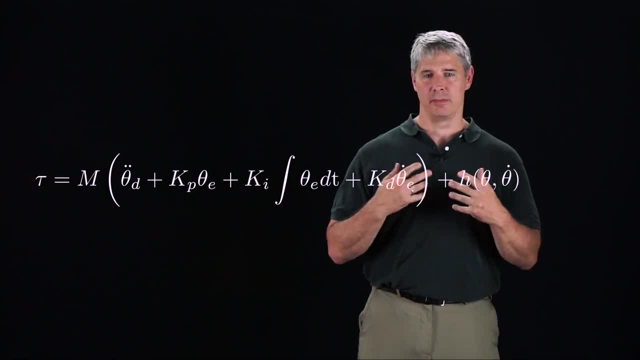 If the model M-tilde and H-tilde is exact, we can remove the tildes in our analysis of the control law. 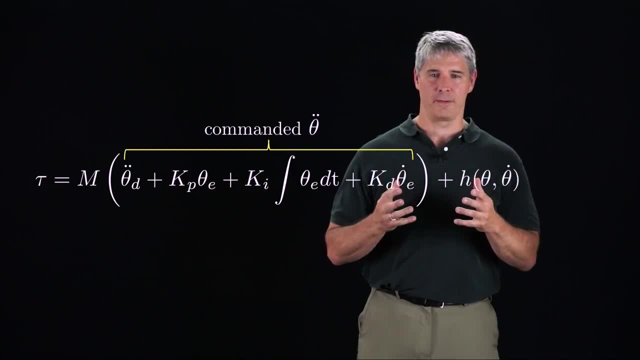 Then the commanded acceleration theta double dot, which is the sum of the feed-forward and feedback terms, is achieved exactly by the commanded torques. The second derivative of the error is theta double dot. This is theta d double dot minus theta double dot. 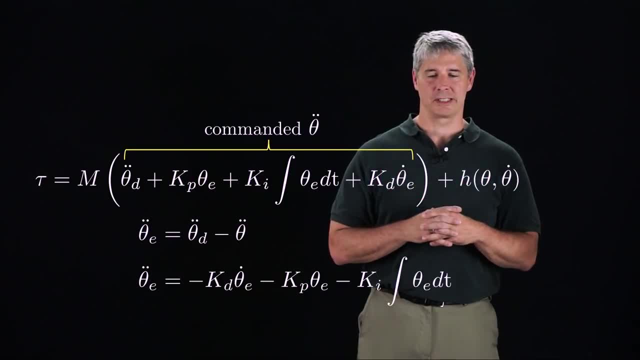 Plugging in the commanded acceleration, the error dynamics can be expressed like this. Taking the derivative, we get this third-order homogeneous differential equation yielding zero steady-state error. 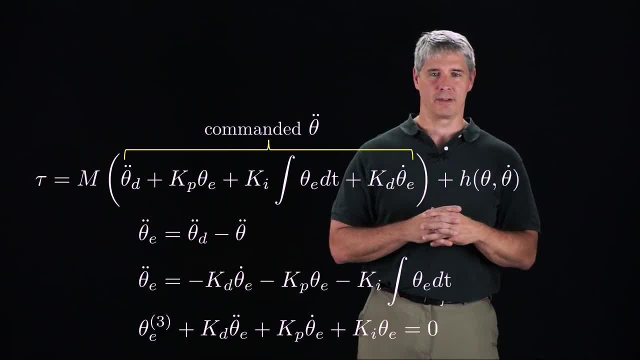 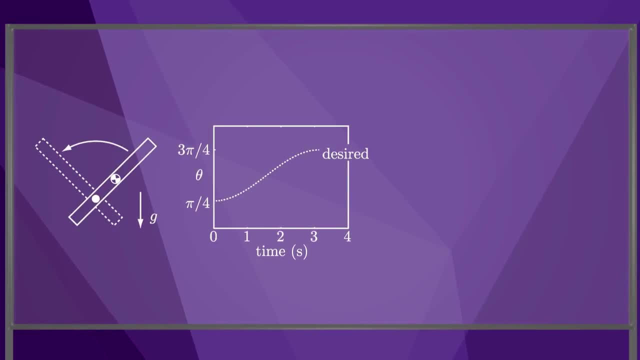 This linear error dynamics applies along arbitrary trajectories of the robot, since the use of the dynamic model effectively linearizes the dynamics. Let's apply the computed torque controller to track the trajectory shown here. 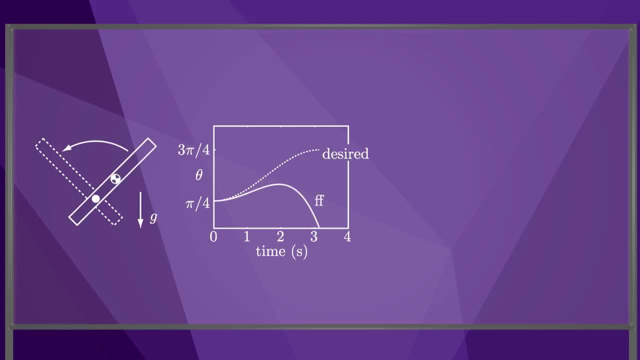 Our model of the dynamics is not perfect, as you can see. You can see from this simulation of the trajectory when using only feed-forward control. 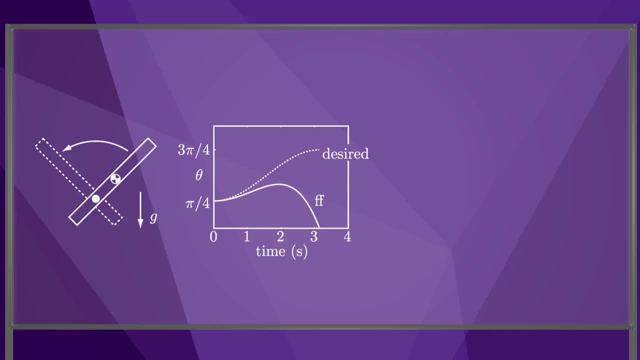 The robot starts out approximately on the trajectory, but over time the actual trajectory diverges from the desired due to error in the model. 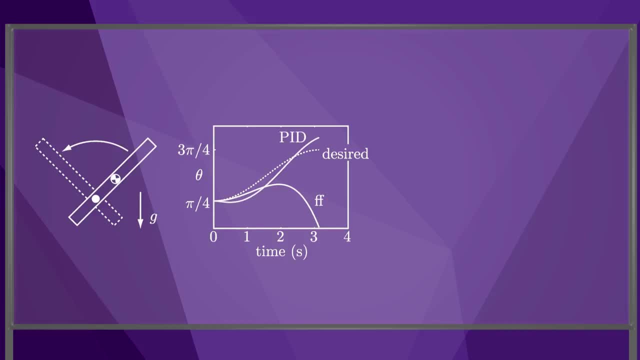 We could instead try a PID controller with no dynamic model. 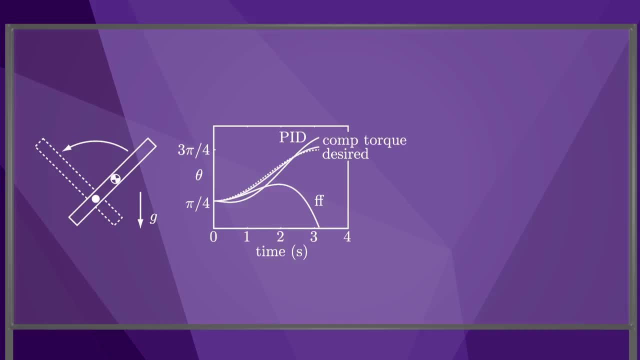 Finally, we could try computed torque, which provides better tracking than either of the other two controllers. We could also look at a standard measure of the control effort exerted by the motor, the time integral of the torque squared. 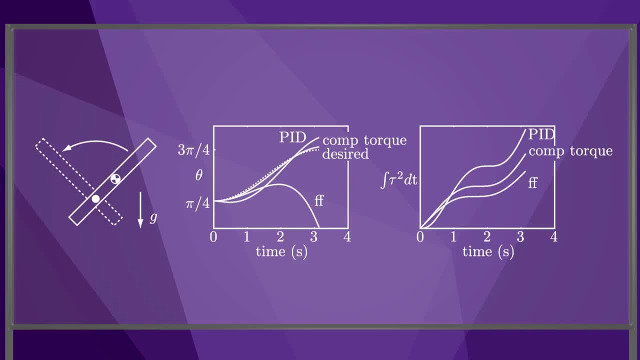 At first, the PID control effort is the lowest, before the error builds up to start driving the torque. Soon, though, the PID control effort exceeds the control effort of the computed torque method. This is typical behavior of the computed torque method. 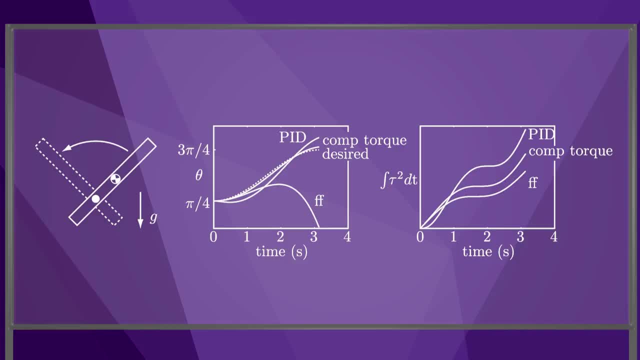 It provides better trajectory tracking than pure feedback control with lower control effort. 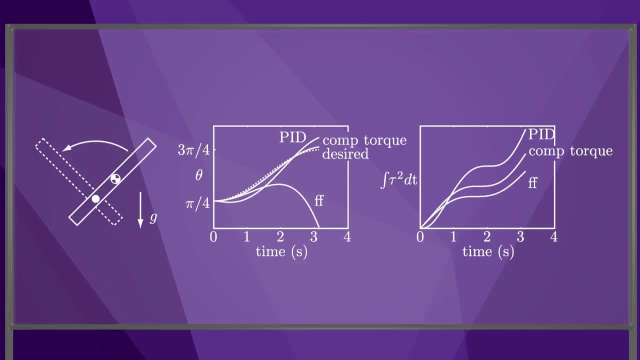 In short, if we have a reasonable model of the robot's dynamics, we should use it in the controller. 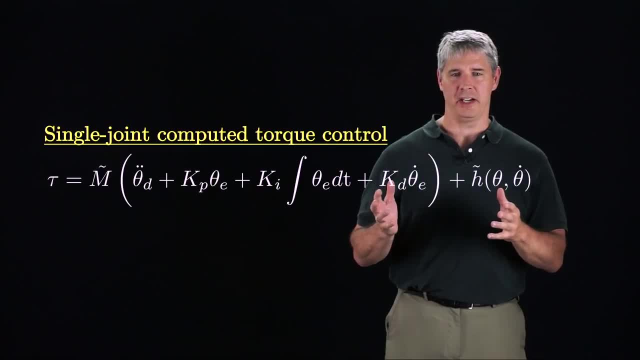 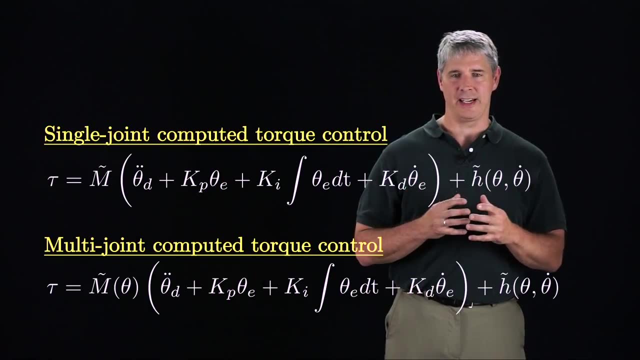 To summarize, the single-joint computed torque control law is given here. This controller generalizes readily to multi-joint robots. The difference is that tau, theta-d, and theta-e are vectors, h-tilde is a vector of Coriolis, gravity, and possibly friction terms, m-tilde is a model of the robot's configuration-dependent mass matrix, and kp, ki, and kd are diagonal matrices, each consisting of a positive scalar times the identity matrix. The linearization of the dynamics provided by the model m-tilde and h-tilde makes each joint have the same stable linear error dynamics. This is a block diagram of the computed torque controller. 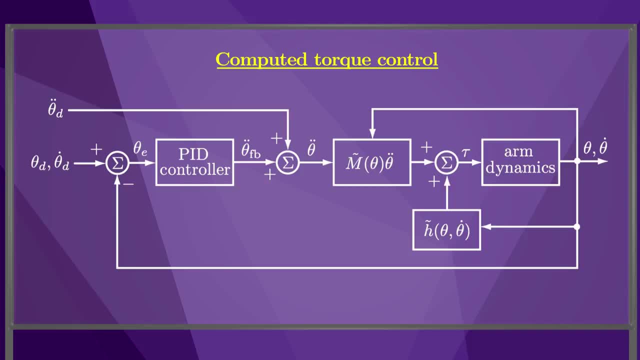 The measured position and velocity of the robot feed back to the PID controller, to the calculation of the m-tilde matrix, and to the calculation of the h-tilde vector. 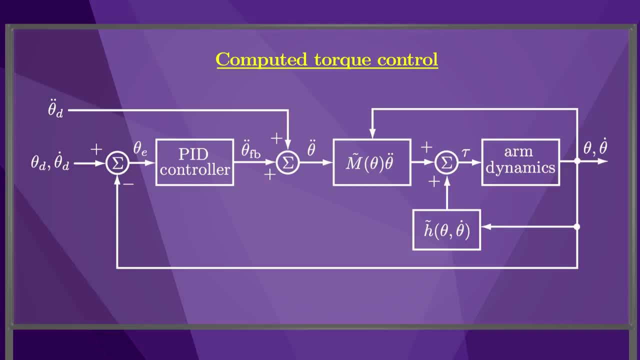 This controller provides good performance when the dynamic model of the robot is reasonably good. If the dynamic model is poor, then using it in the controller could actually hurt performance compared to a model-free feedback controller. Also, evaluating the mass matrix and h-vector could be computationally intensive for real-time control. For this reason, simpler versions of this control law are common. For example, PD feedback control plus gravity compensation can provide good performance, and it is much less computationally expensive to evaluate a model of gravitational torques than it is to compute a full dynamic model. 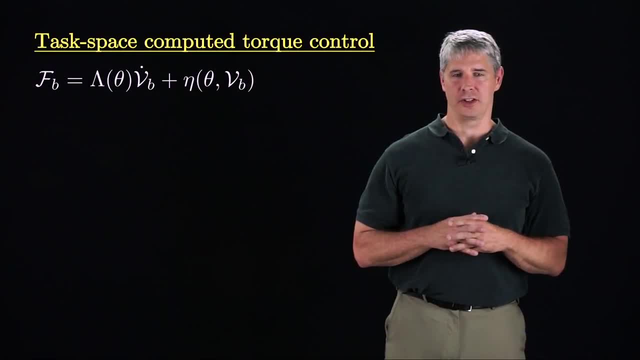 Finally, we could express the computed torque control law in terms of the task space dynamics of the robot derived in Chapter 8. 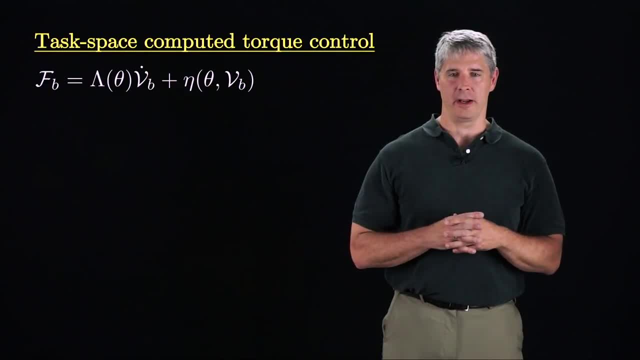 The end-effector wrench FB, expressed in the end-effector frame, equals the end-effector mass matrix lambda times the end-effector acceleration VB-dot 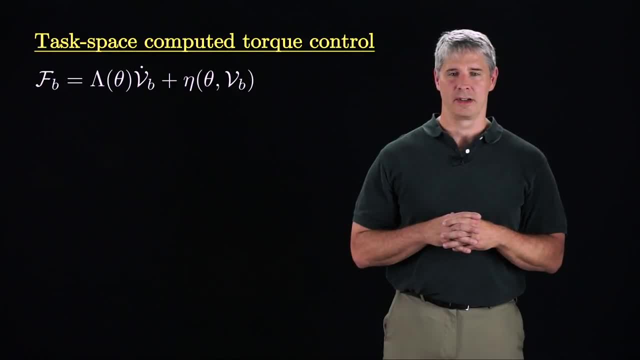 plus the wrench eta due to Coriolis and gravity terms. Our dynamic model is lambda-tilde and eta-tilde. 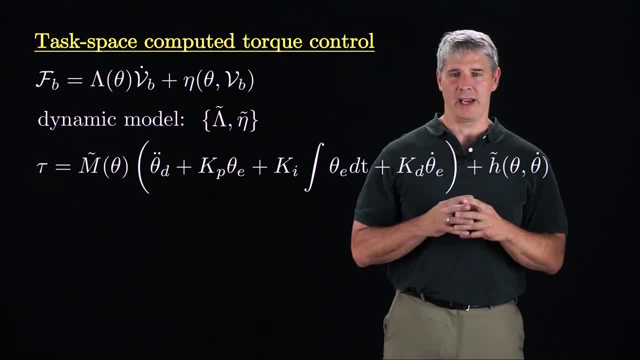 Recalling the joint-space computed torque control law, by analogy, rewrite the task-space computed torque control with FB, lambda-tilde and eta-tilde, replacing tau, m-tilde and h-tilde, respectively. The analog to the feed-forward acceleration theta-d-double-dot is the time derivative of the desired twist, VD-dot.